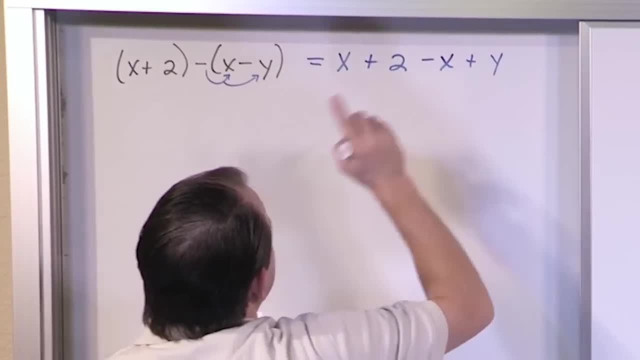 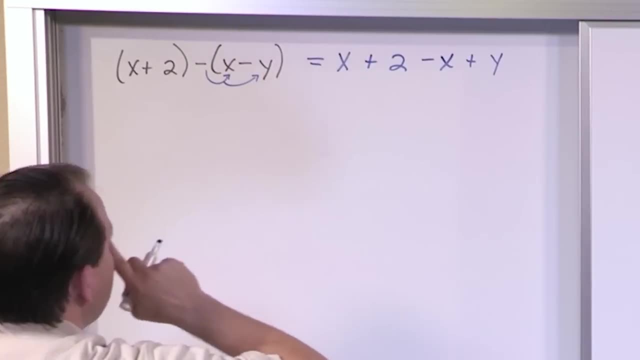 1 times negative y. It's just going to be positive y. Don't forget negative times. negative is positive. So you need to make sure and do that When you distribute this sign in. you need to make sure and get these signs right Now can we simplify this Well? 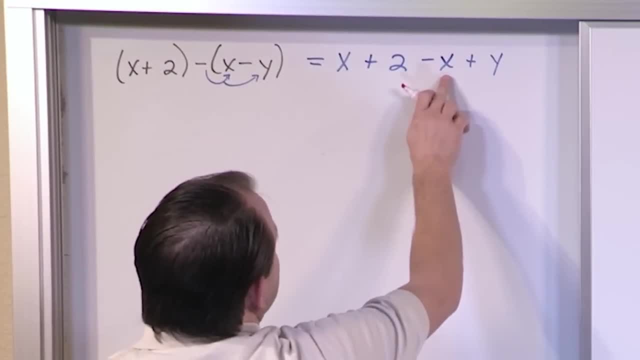 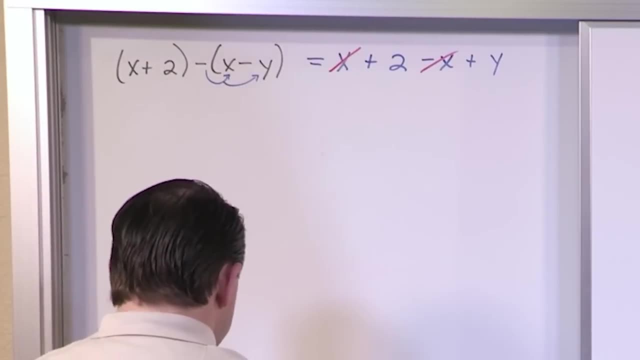 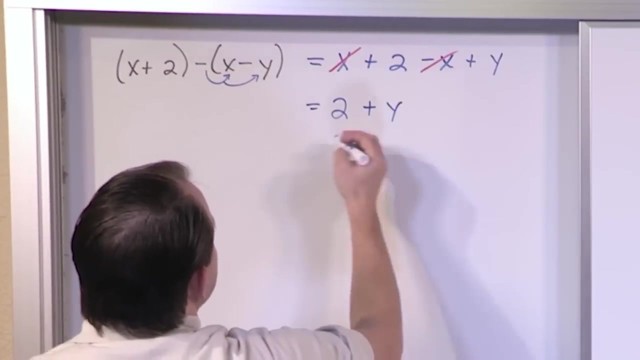 I see right away that I have an x here and a minus x here. So when I take x and subtract x, it's going to give me 0, so they're going to basically disappear, And then what I'm left with is 2, and then over here plus y. Usually you like to write the variable first. 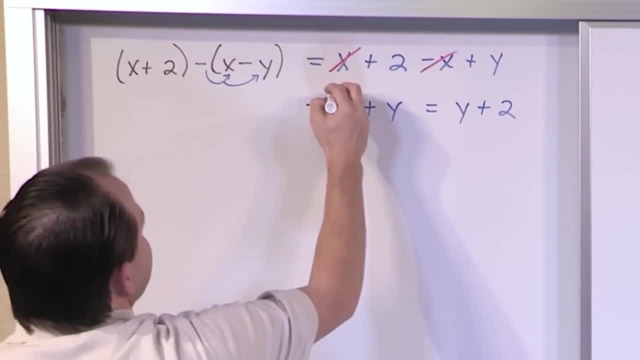 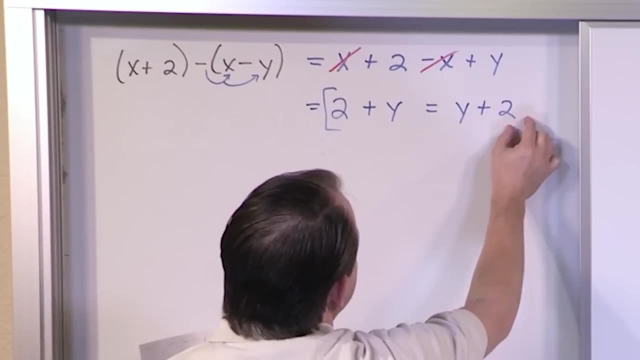 so it would be y plus 2.. Same thing: 2 plus y is the same as y plus 2.. And that is the final answer. You can't simplify this anymore, because here I have y's that I'm talking about and here I'm just having numbers. There's no y here, so I can't actually. 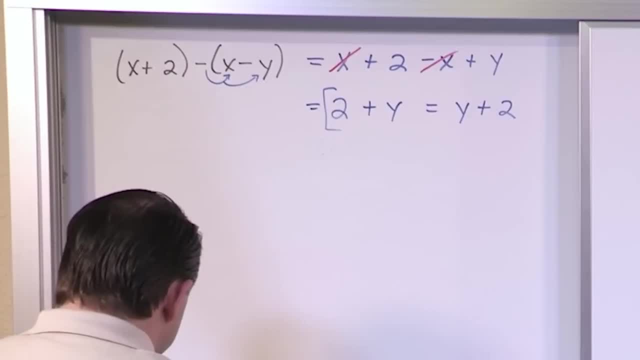 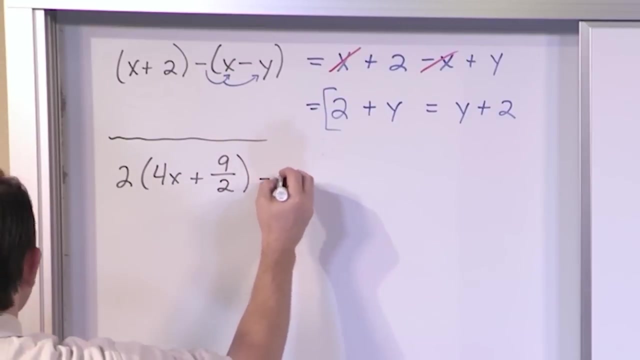 add those anymore. So that is the final answer. Now let's flex our muscles a little bit, And I think you've got the basic idea of how to do this. Let's start rolling in some of our other skills: 2 times 4x plus. here's a good old fraction: 9 halves minus 3x plus. 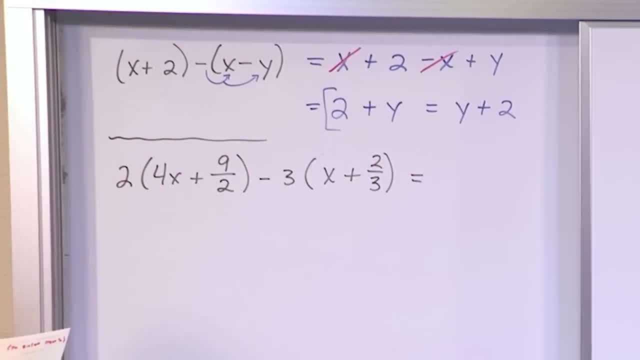 2 thirds. I told you, fractions would never leave your side when you're dealing in algebra, And it's better just to tackle it head on and understand it rather than hide from it. So here we have some stuff inside of parentheses. Here we have some stuff inside of parentheses. 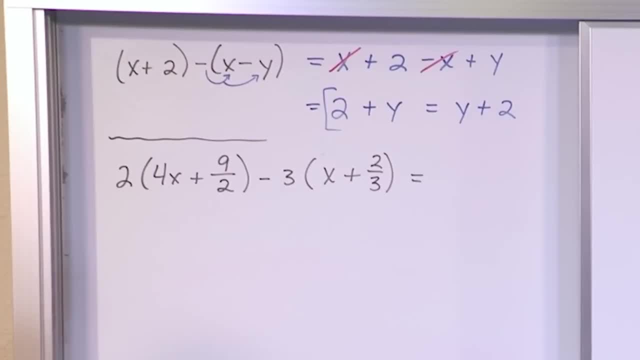 We have fractions everywhere. So the first thing you want to do if you want to try to simplify it is go in here and try to simplify this, But you realize you can't, because this is x's we're dealing with and there's no x there, So we can't actually add this Same. 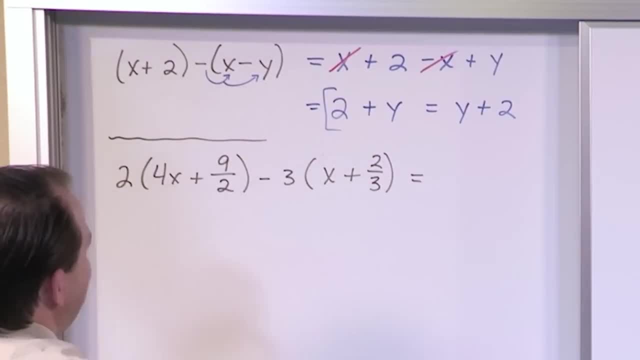 problem here. We don't have any x's over here, So we can't actually add them together. So we're kind of stuck there. But we notice that we have a number outside of this parentheses, and we have a number outside of this parentheses. 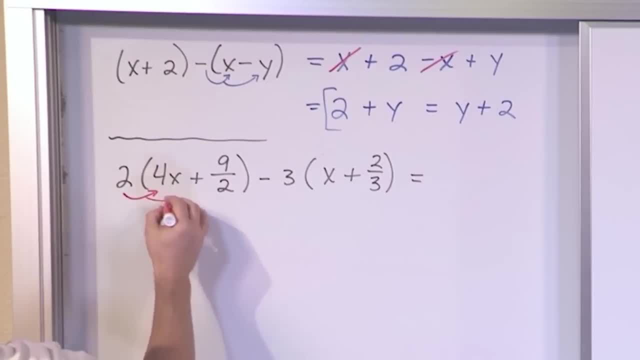 So we're going to be able to distribute, for instance, the 2 into here and into here, and we'll distribute the negative 3.. Don't forget, it's negative. because of this, We'll distribute that into the second set. So how do we distribute a 2 in? Well, it's going to be 2 times 4x. 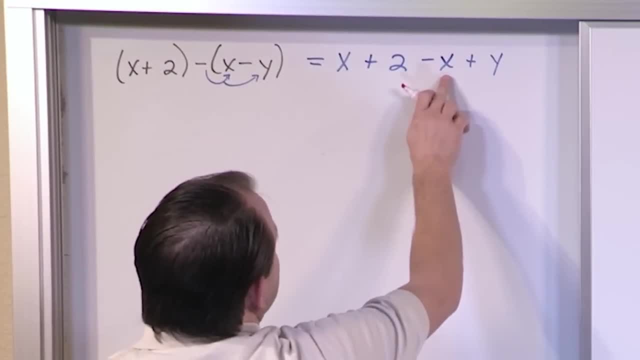 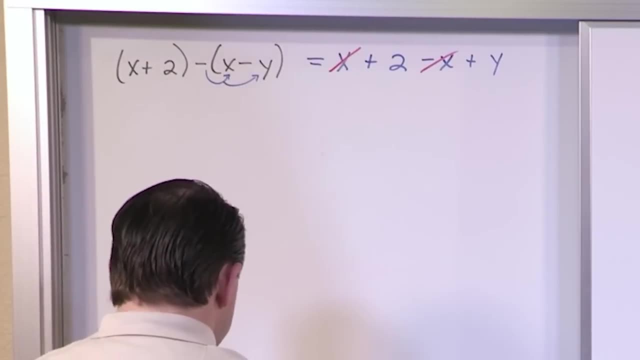 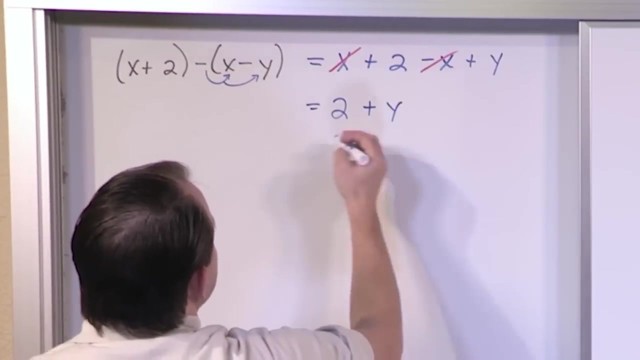 I see right away that I have an x here and a minus x here. So when I take x and subtract x, it's going to give me 0, so they're going to basically disappear, And then what I'm left with is 2, and then over here plus y. Usually you like to write the variable first. 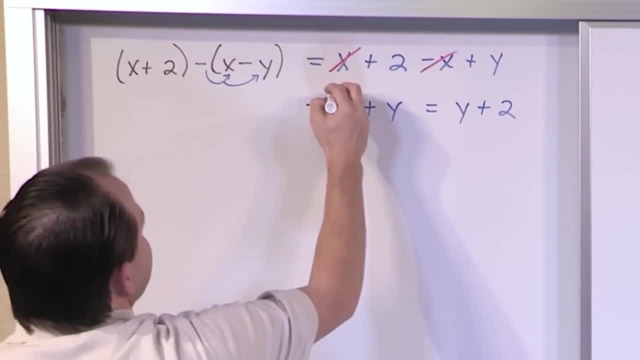 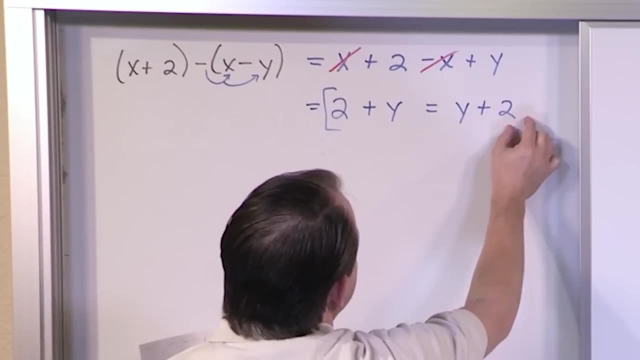 so it would be y plus 2.. Same thing: 2 plus y is the same as y plus 2.. And that is the final answer. You can't simplify this anymore, because here I have y's that I'm talking about and here I'm just having numbers. There's no y here, so I can't actually. 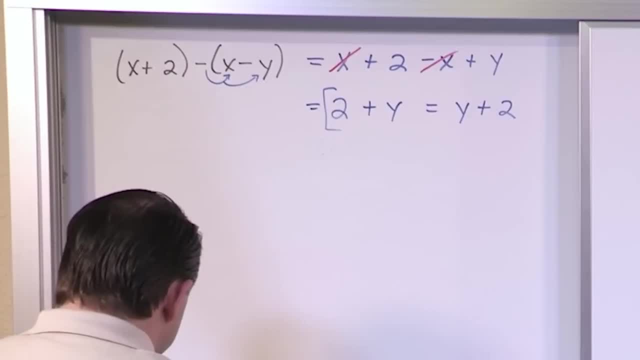 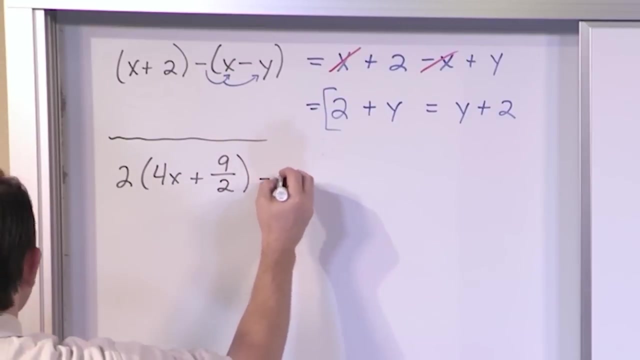 add those anymore. So that is the final answer. Now let's flex our muscles a little bit, And I think you've got the basic idea of how to do this. Let's start rolling in some of our other skills: 2 times 4x plus. here's a good old fraction: 9 halves minus 3x plus. 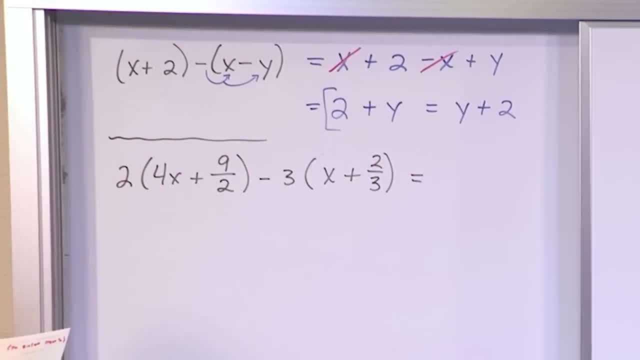 2 thirds. I told you, fractions would never leave your side when you're dealing in algebra, And it's better just to tackle it head on and understand it rather than hide from it. So here we have some stuff inside of parentheses. Here we have some stuff inside of parentheses. 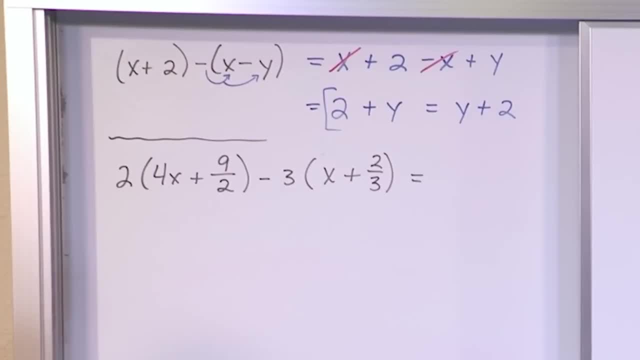 We have fractions everywhere. So the first thing you want to do if you want to try to simplify it is go in here and try to simplify this, But you realize you can't, because this is x's we're dealing with and there's no x there, So we can't actually add this Same. 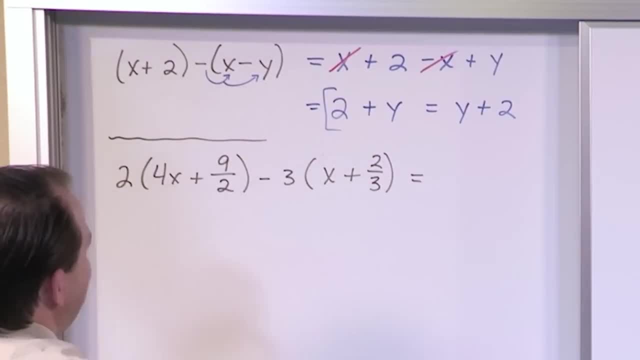 problem here. We don't have any x's over here, So we can't actually add them together. So we're kind of stuck there. But we notice that we have a number outside of this parentheses, and we have a number outside of this parentheses. 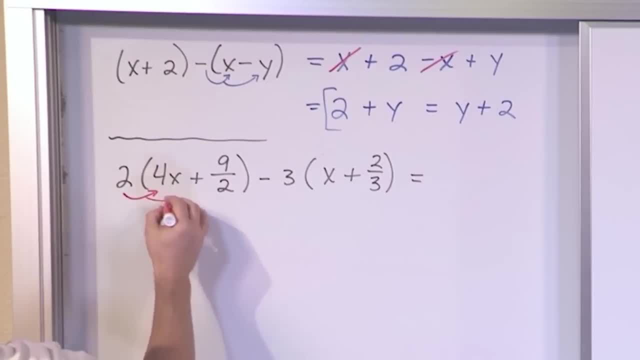 So we're going to be able to distribute, for instance, the 2 into here and into here, and we'll distribute the negative 3.. Don't forget, it's negative. because of this, We'll distribute that into the second set. So how do we distribute a 2 in? Well, it's going to be 2 times 4x. 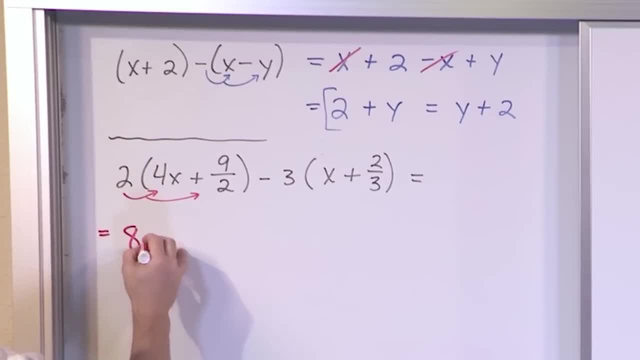 What's 2 times 4x? Well, you multiply the numbers and you're going to get 8 x's. All right, When you're multiplying things together like a number times 4x, you multiply the number and you carry the variable down, Because this is like 4 pencils right. X could represent. 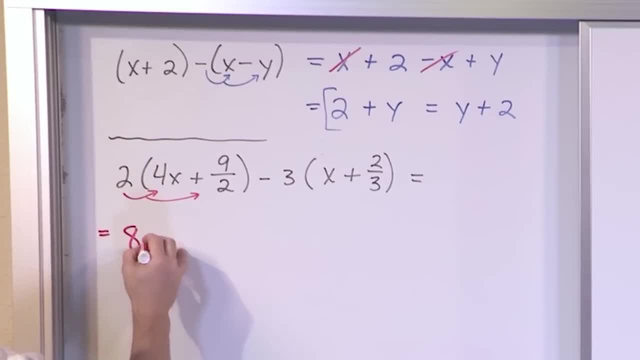 What's 2 times 4x? Well, you multiply the numbers and you're going to get 8 x's. All right, When you're multiplying things together like a number times 4x, you multiply the number and you carry the variable down, Because this is like 4 pencils right. X could represent. 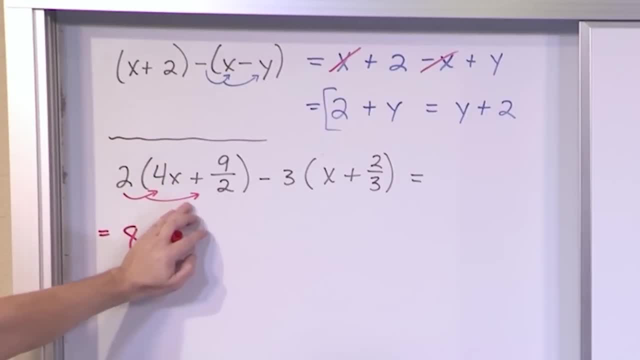 whatever pencils. So 2 times 4 pencils. if you just put 8, it wouldn't make sense. You have to represent what you're talking about. So it's 8 pencils here, So 8x, for instance. 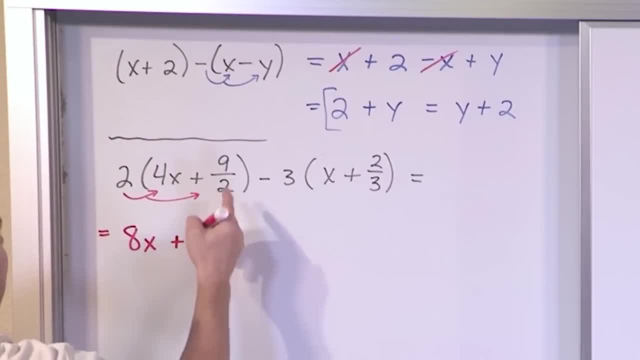 And then we'll have- let me take this one step at a time- 2 times 9 halves, And we'll just deal with the actual multiplication later. But you should understand that we're multiplying 2 times 9 halves, All right. And then over here we have negative 3x, because 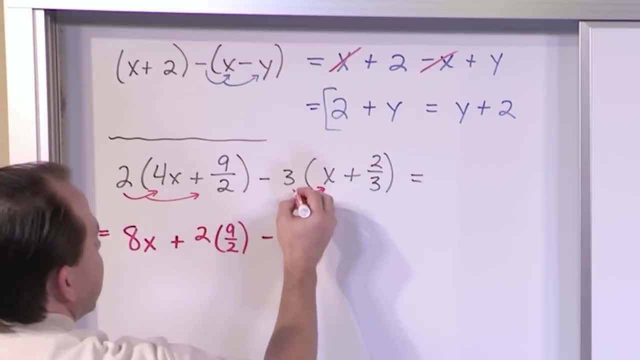 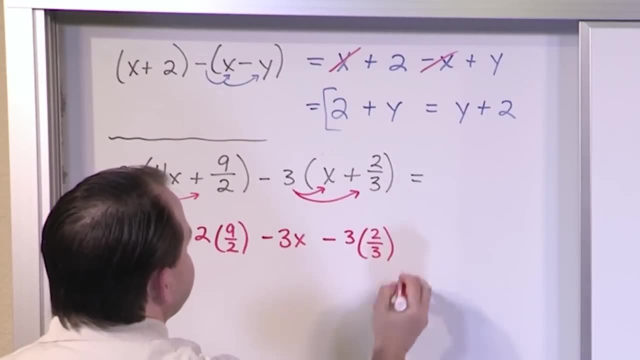 we're multiplying negative 3 times x And then over here we're multiplying negative 3 times this guy. So we'll carry the negative sign negative 3 times 2 thirds. So that's what we have for this part here. Now the thing I want to point out to you here, and kind 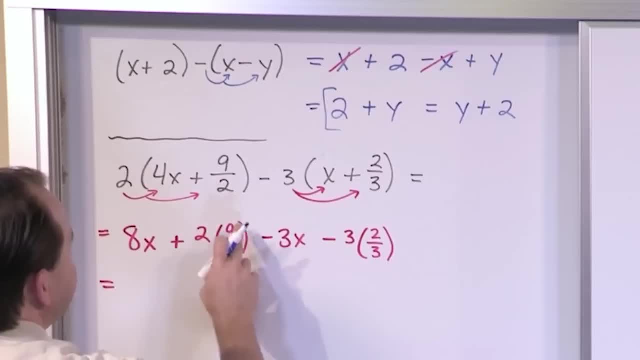 of why this problem was constructed this way. we have a 2 and we're multiplying by 9 halves. So don't forget any time you're multiplying by a number, it's kind of like saying 2 over 1, basically. So it's kind of like you can imagine this fraction multiplying by this. 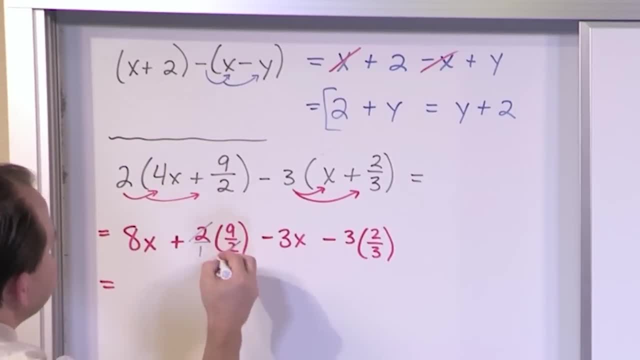 fraction. You have a 2 on the top and a 2 on the bottom, Though they're basically going to cancel, They're going to divide out. basically, 2 divided by 2 is going to give you 1. It's. 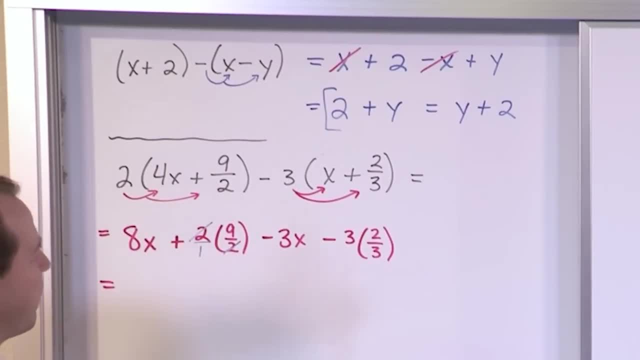 going to disappear Any time. you have something on the top and the bottom of a fraction that's going to happen And you have exactly the same thing going on over here. The 3 is going to cancel with the 3.. I mean, when you think about it, 3 times 2 is 6.. 6 divided by 3 is 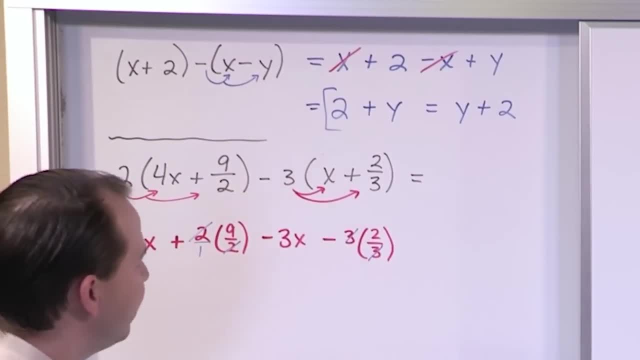 2.. So if you actually did the multiplication, you're still going to get 2.. Same thing that you get by just canceling them out. That's what you're going to get there. So, continuing on, you'll have 8x plus. after this cancellation, you just have a 9 there, minus 3x minus after. 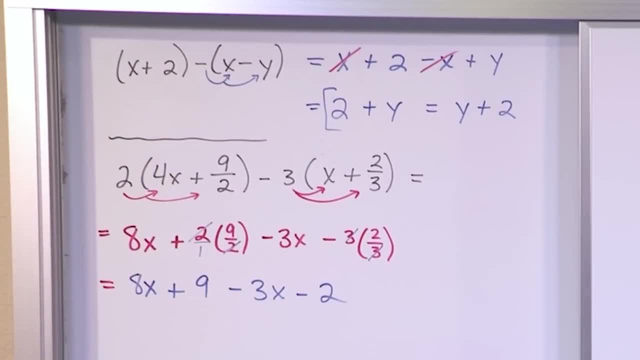 this cancellation. you just have a 2 there. All right. now we're finally to the point where we can add some terms together. We have 8x's here and we have minus 3x's here, So 8 minus 3 is 5.. 5- what 5x's? 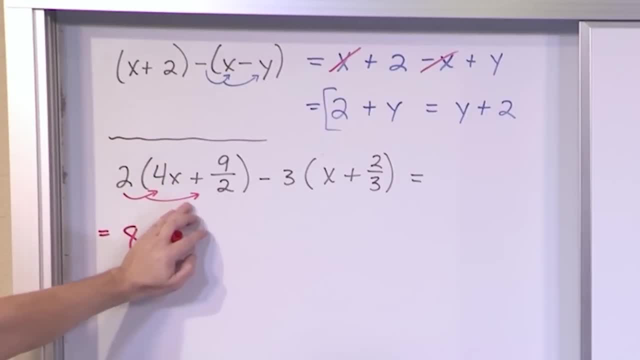 whatever pencils. So 2 times 4 pencils. if you just put 8, it wouldn't make sense. You have to represent what you're talking about. So it's 8 pencils here, So 8x, for instance. 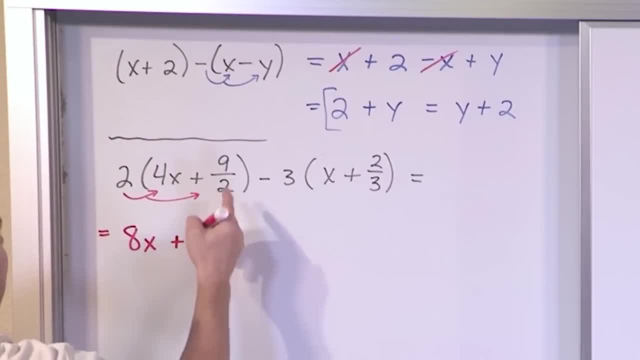 And then we'll have- let me take this one step at a time- 2 times 9 halves, And we'll just deal with the actual multiplication later. But you should understand that we're multiplying 2 times 9 halves, All right. And then over here we have negative 3x, because 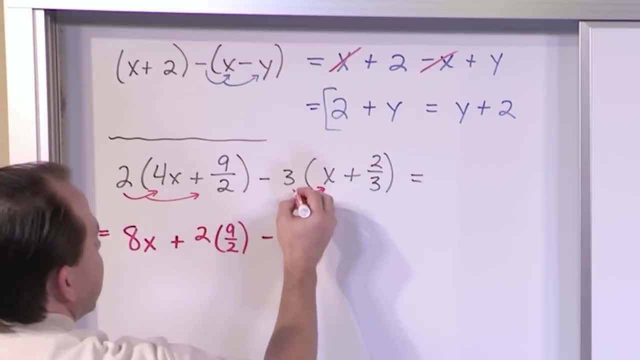 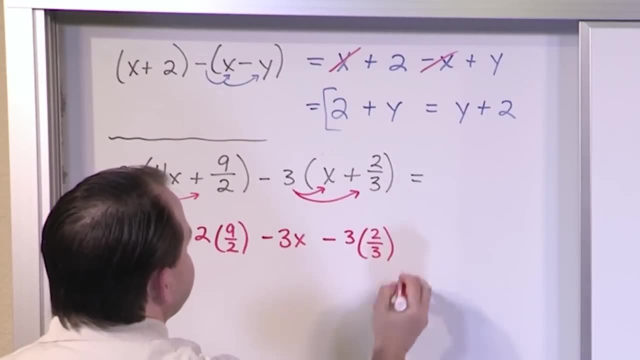 we're multiplying negative 3 times x And then over here we're multiplying negative 3 times this guy. So we'll carry the negative sign negative 3 times 2 thirds. So that's what we have for this part here. Now the thing I want to point out to you here, and kind 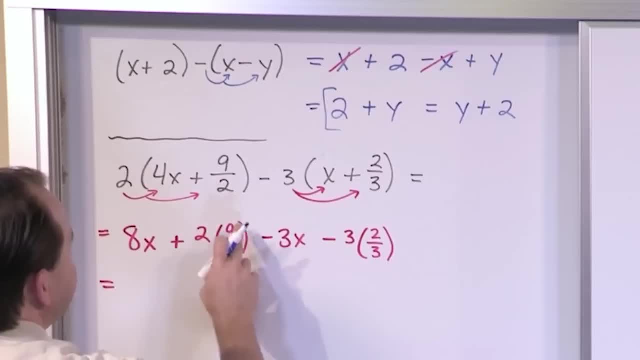 of why this problem was constructed this way. we have a 2 and we're multiplying by 9 halves. So don't forget any time you're multiplying by a number, it's kind of like saying 2 over 1, basically. So it's kind of like you can imagine this fraction multiplying by this. 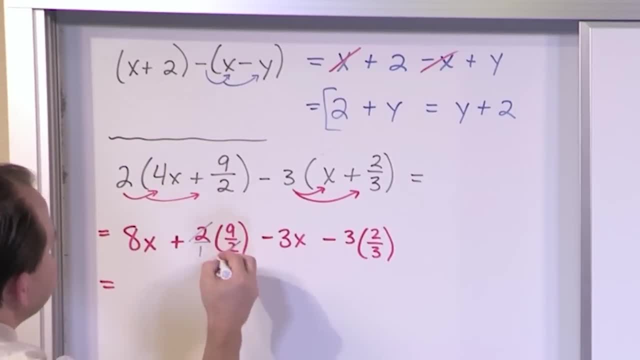 fraction. You have a 2 on the top and a 2 on the bottom, Though they're basically going to cancel, They're going to divide out. basically, 2 divided by 2 is going to give you 1. It's. 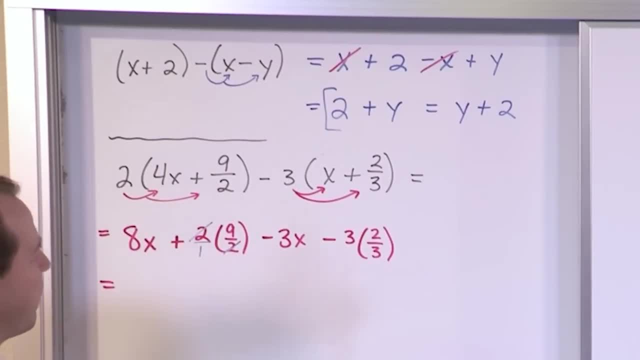 going to disappear Any time. you have something on the top and the bottom of a fraction that's going to happen And you have exactly the same thing going on over here. The 3 is going to cancel with the 3.. I mean, when you think about it, 3 times 2 is 6.. 6 divided by 3 is 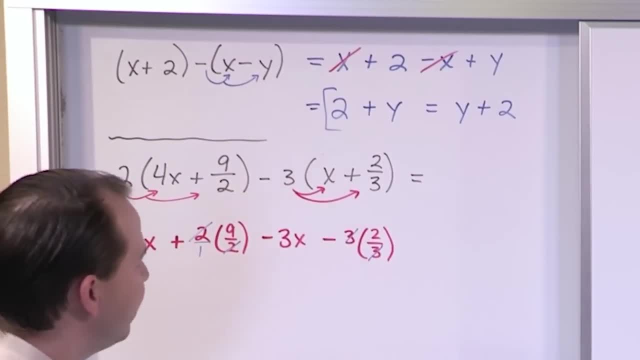 2.. So if you actually did the multiplication, you're still going to get 2.. Same thing that you get by just canceling them out. That's what you're going to get there. So, continuing on, you'll have 8x plus. after this cancellation, you just have a 9 there, minus 3x minus after. 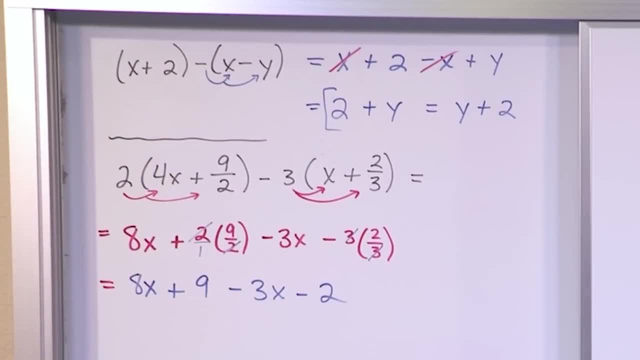 this cancellation. you just have a 2 there. All right. now we're finally to the point where we can add some terms together. We have 8x's here and we have minus 3x's here, So 8 minus 3 is 5.. 5- what 5x's? 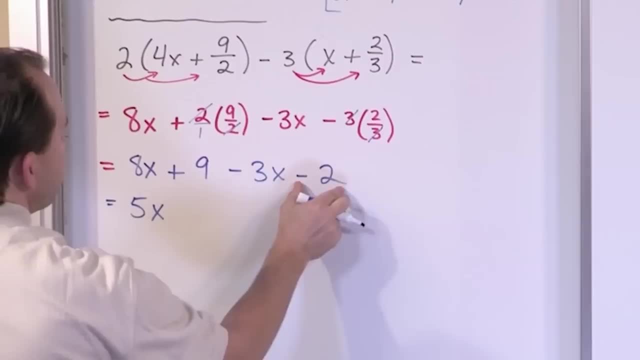 You have to carry the variable along, And then we have some numbers: 9 minus 2 is positive 7. So it's 5x plus 7. And that is the final answer. All right, so the only thing that was even a little bit tricky about this is we had to distribute 2 times from the numbers.